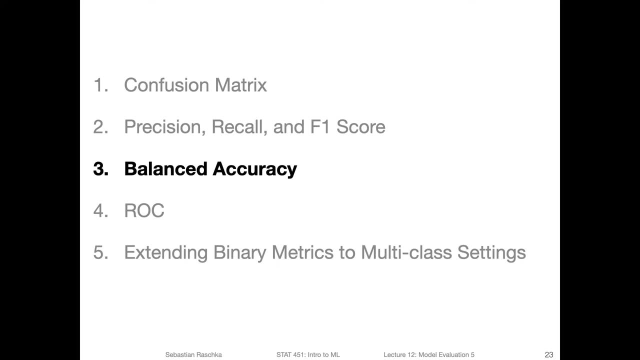 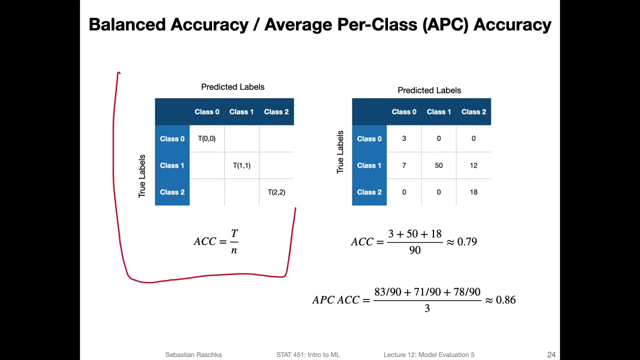 All right, let's now talk about the balanced accuracy, which is helpful if we have class imbalance problems. That means if one class has more labels than another class. So here's an example. I'm showing you a confusion matrix for a multi class classification problem. 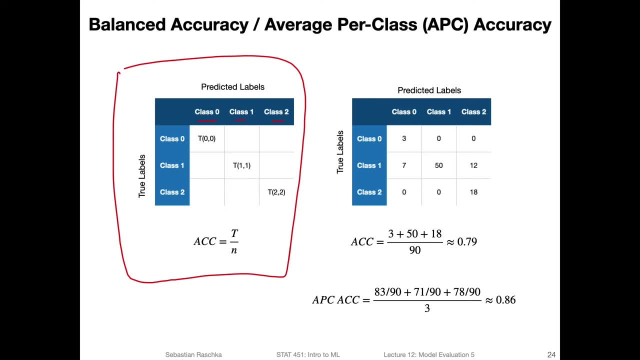 So where we have class zero, class one and class two, three classes, And you can think of it as, for example, iris setosa, iris versicolor and iris virginica flowers, And typically we would compute the prediction accuracy by summing over the diagonals here and then dividing by the total. 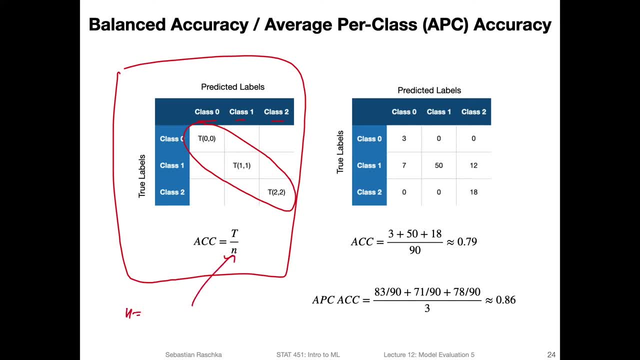 number of examples. So n is the data set size in this case. So if I have a concrete example, like shown here on the right hand side, so on here what I have is three labels from class zero, then seven, 69 labels from class one. So if you would add up all in the row that 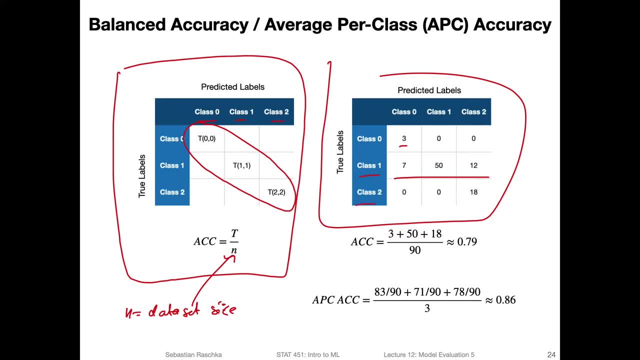 other class one examples and then we have 18 class two examples. So in this case we have a class imbalance problem. you can see there are 69, three and 18.. So there are more examples from class one than from class zero and class 18.. If we would compute the regular accuracy we would 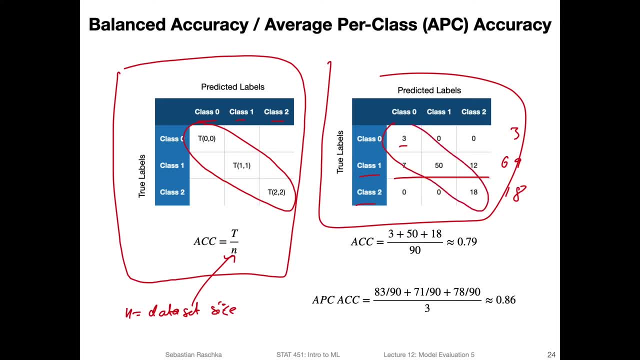 compute it by just something over diagonal and then by the total number of data points. Here it's: the total number of data points is 90. And we would get approximately 80%. So now it's emphasizing the middle class, low class, one right because it's the most data points. if, for example, our 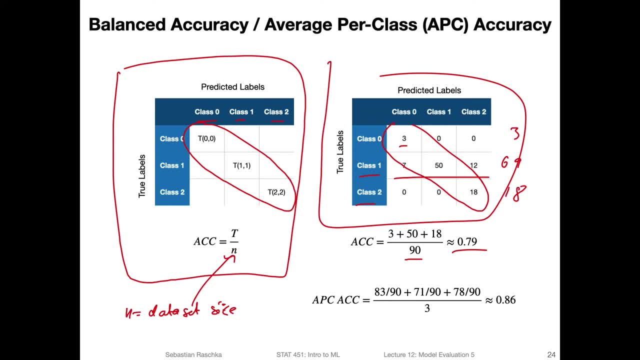 classifier for class zero, instead of predicting them correctly. let's say it predicts zero here, then a two here and the one here. If the prediction is like that, and this one will change to zero, but it will not affect really our accuracy. So the average per class. 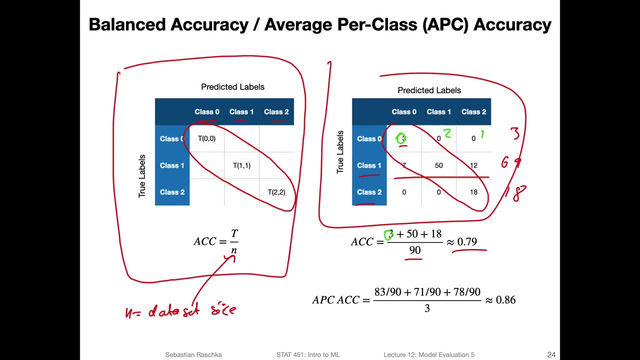 accuracy aims to kind of have a more balanced view on that. So each class counts equal, equally. So here in this case, on how it's computed, it's computing the accuracy for each class, in this case, So the accuracy for class zero versus all the other classes. how is that? 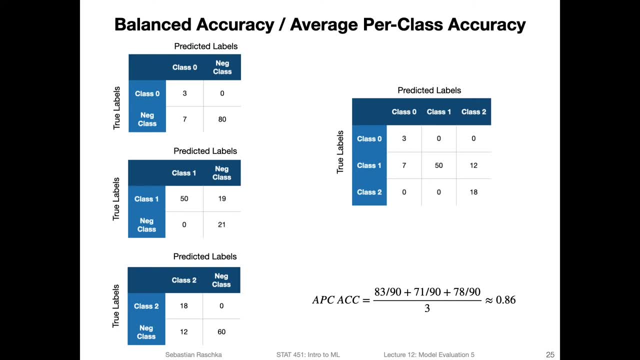 computed, So it's a little bit complicated to look at it just like this, which is why I made a separate slide, Because what we are doing is we are computing three accuracies and averaging over the three. So how do we compute each accuracy? So each one? you can think of it as a binary. 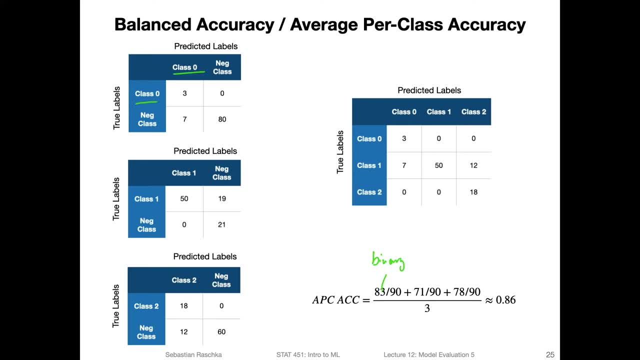 accuracy. So let's maybe take a look at class zero first. So what we do is we regard class zero as the positive class And in all the other classes we summarized as the negative class. So we will. if we take a look at the right here, we will take a look at this window here. So we have 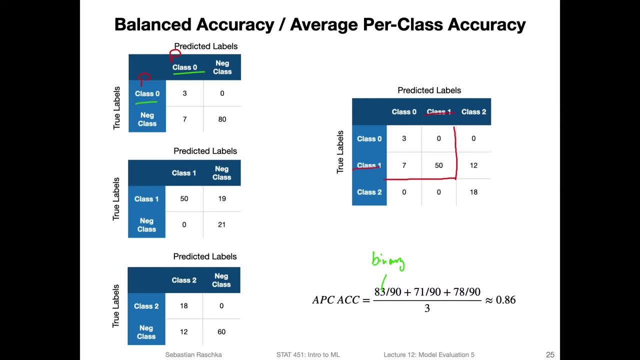 class zero And then for class one, we will now call them: So this is a positive class And this is class one will be the negative class. So what about class two? we have to pull or combine class 001? class two- into the negative class, So both other classes. 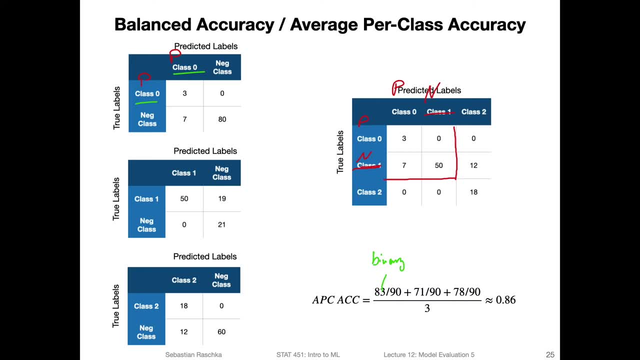 will become the negative class. So what we're doing is we are merging them into here, So this one will become at then. So we will make this binary classification problem. So why is that done like this? So I mean, if we look at the number, 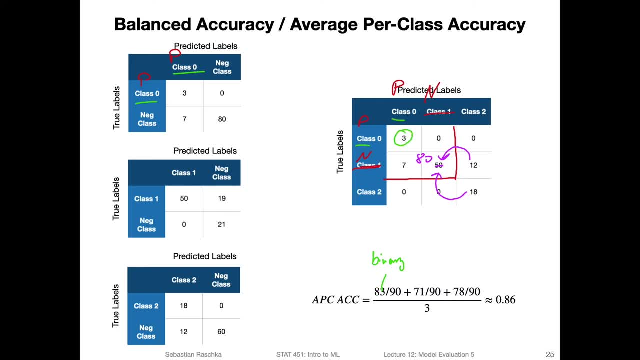 of classes zero predicted a zero. the number doesn't change, it's still three. If we take a look at the examples of true class zero that are classified as not zero, it's still zero because we are pulling this number in- actually two, but it. 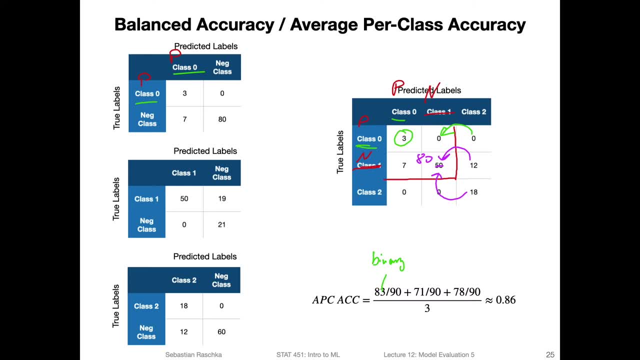 stays zero, right. So in this case nothing really changes here. And then for the other classes here that are predicted as class zero, we pull this one in, but it's zero, So also, this one doesn't change. it's still only seven of. 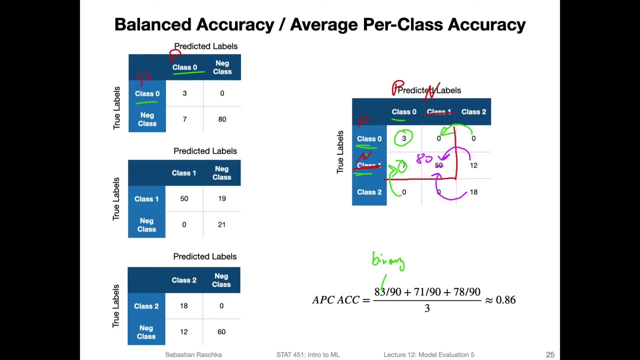 the negative classes are predicted as class zero, However, yeah, all the other ones change. So this is, for example, for class zero, if I erase that, and we take a look at So, by the way. so here now the number of true positives is: 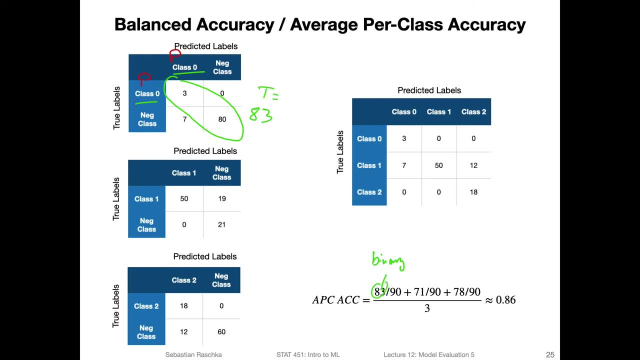 83. Which is why we have it here. right? This is where the number comes from. But now let's do the same thing for class one. So for class one. now we take a look at the example where class one- let me use the. 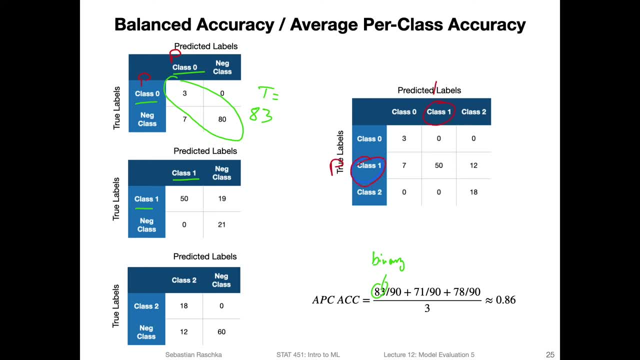 red color. here again, class one becomes the positive, And now class zero and plus two become the negatives. So we have to combine them again. So how do we combine them? Can, for example, maybe just take take those here, So, and then we would combine. 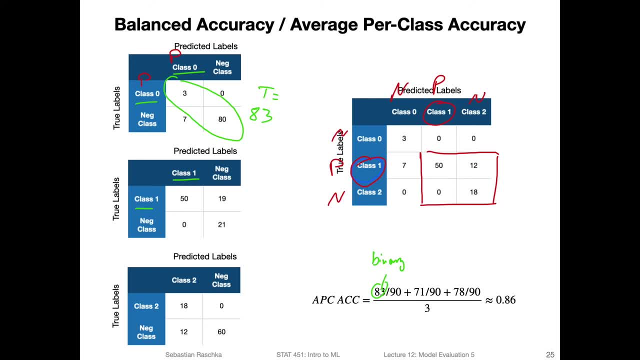 them by, yeah, merging, merging them again. So class one predicted as class one, this doesn't change really, But then for example, class one, So these would be basically merged into this one. because now, if we consider this as the, 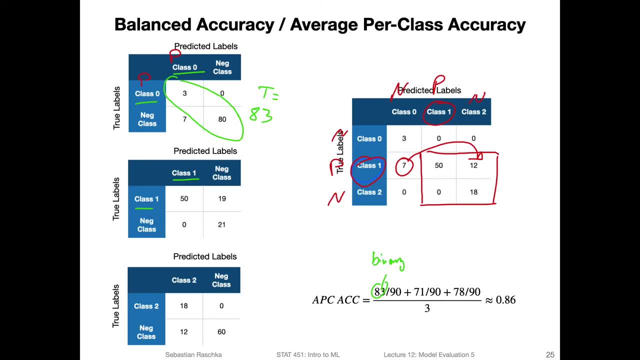 positive class. so how many? how many of the true class- sorry, the how many of the true class ones- are not predicted as class one. this is actually both. this class is seven and 12. So we will, if we look at this window, we will put this as a 19. And so 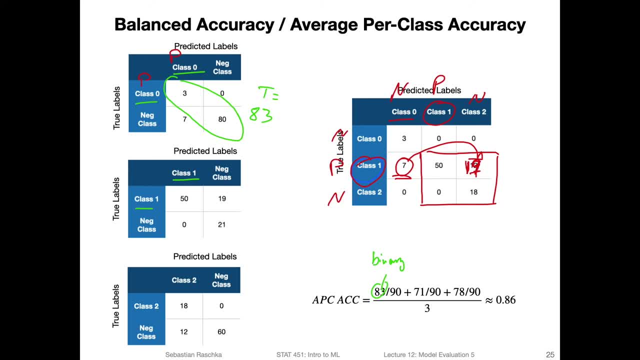 and how many true negatives do we have? So the true negatives are class one- sorry, class two predicted as class two and class zero predicted as class zero. So these are the true negatives. So we are adding the three to this one, So we get 21 here. 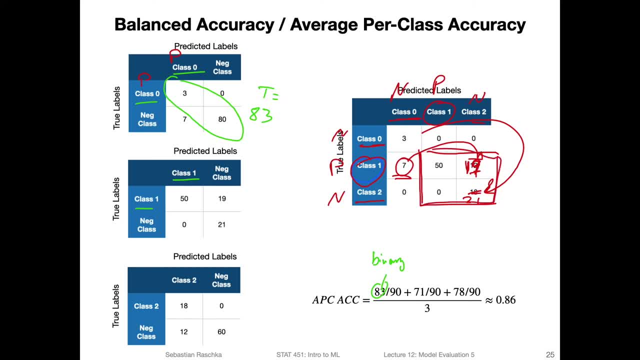 And then again, if we have this window and we take the diagonal, this is 71. Here, this is where this number comes from, And then we can repeat the same game for class two, which I'm thinking you can do by your own, because otherwise it will probably be. 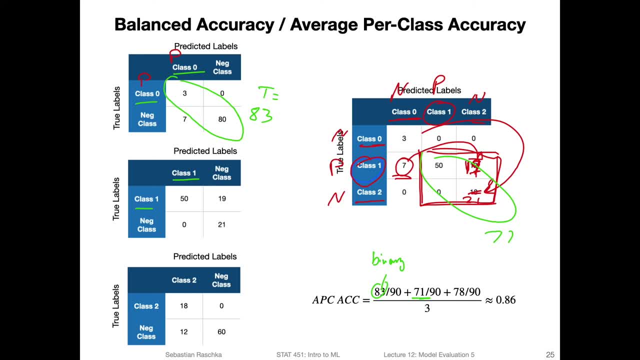 too much erasing here and just doing the same thing as at the time. So in that way it's maybe a good exercise, because there might be an exam question like that, So maybe you can practice this with class two here. Alright, so then, how do we do that in Python? So yeah, this is. 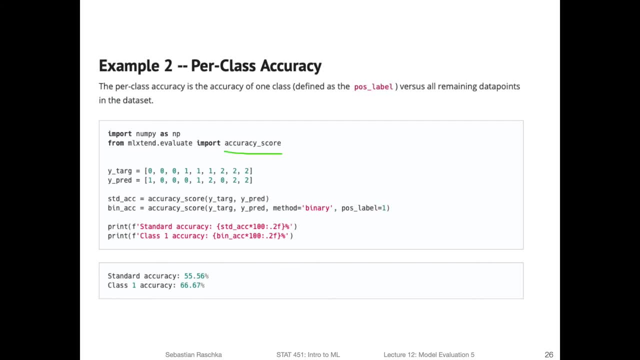 what can be implemented using the accuracy score from ML extend. So the ML extend accuracy score fundamentally look, works the same way as psychic learns, but it has this extra, extra functionality for computing the binary accuracy, which is the binary raising the accuracy, like I showed you. 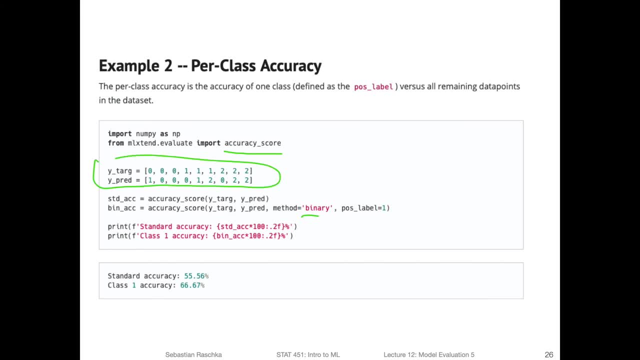 before. So here I don't use a concrete classifier, just a toy example of the true labels and the predicted labels. And then here that's the standard accuracy score. In this case it's 55.56.. And then we have three classes. 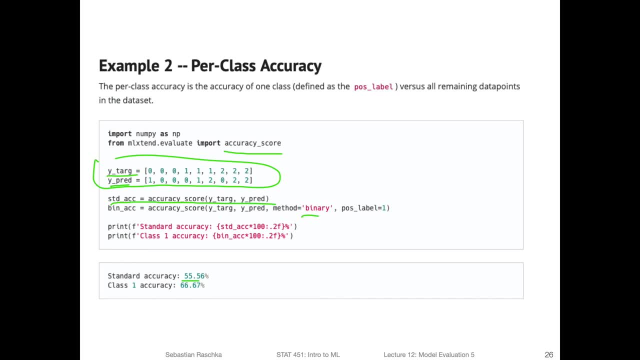 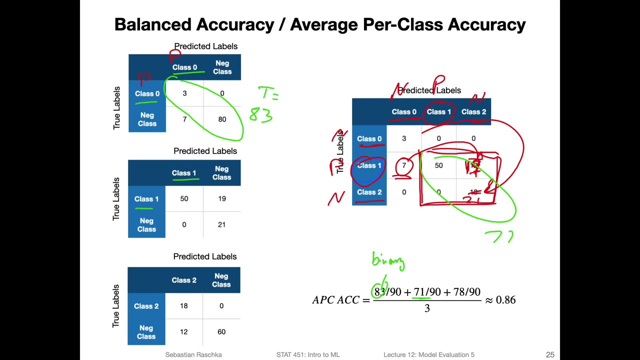 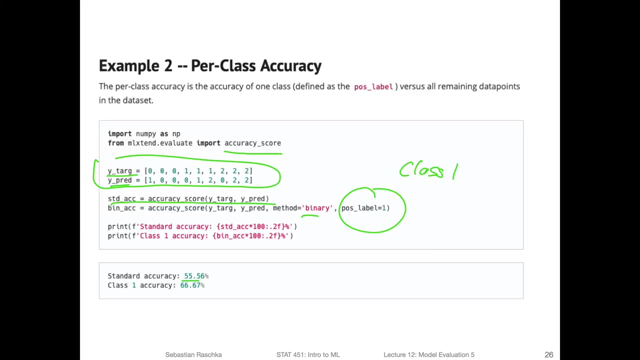 here if I want to compute the binary classification accuracy for class one as the positive label. So this would be then equivalent to to this one where class one is the positive label and everything else is the negative class. you can specify it by specifying the method as binary. 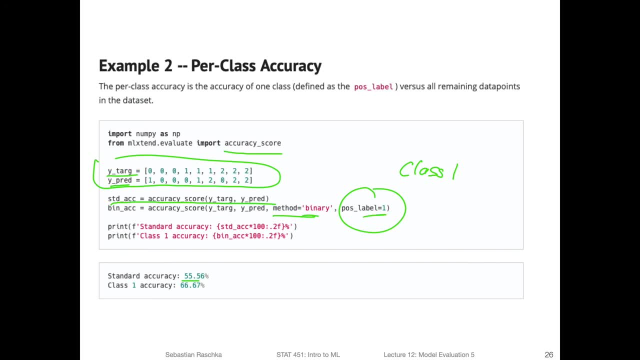 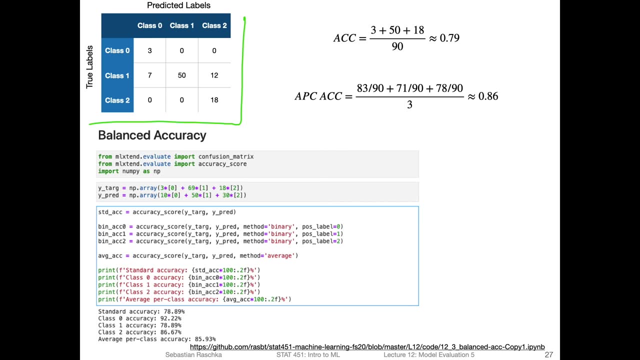 And the positive label is one, and you can do the same thing with zero and two. So this is what I've done here. So here this is the confusion matrix that I showed you two slides ago. Here again for reference, the accuracy and the average per. 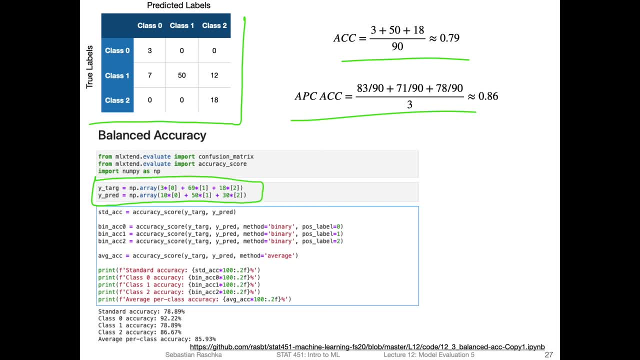 class accuracy. Here I'm just recreating this confusion matrix. I could have maybe visualized it. So if you call confusion matrix on these two arrays, what you would get is this confusion matrix. So here for reference, that's the standard accuracy score. 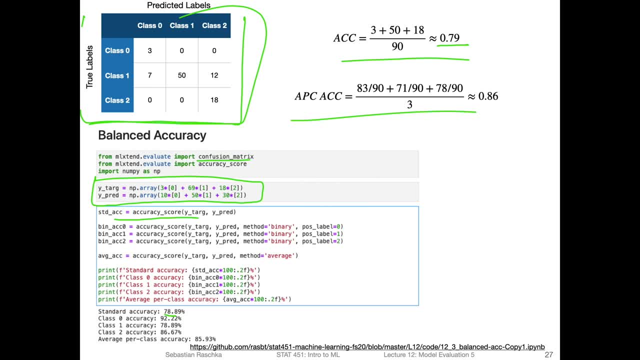 which is 78.89.. So average is 79.. And here I'm computing these binary accuracies which correspond to these ones here. So just for reference, these are the binary accuracy, So you can see them here: approximately 92%, 78.8% and 86.68%, And 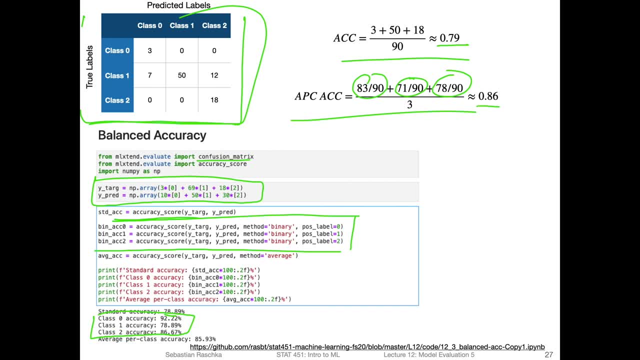 if you would average those, what you would get is approximately 86%, So you can just add them up and divide by three, and then you should get the 86%. However, alternatively, you can make your life easier. just use average as the method here, So it will. 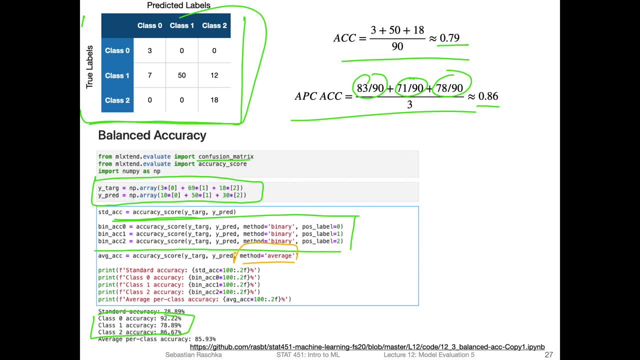 already do it for you, So this one will compute the average per class, also called balanced accuracy. If you want to get this as a code example to play around with that, you can find it on GitHub here. So yeah, this was the balanced accuracy average.